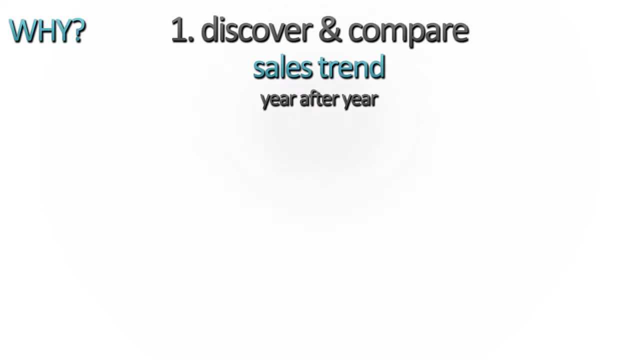 trend and compare it year after year with the market trend, with the competitor's trend. Then if you discover any differences in this comparison, you have to examine in which year and why your sales channel, prices, product quantity, customer service, payment methods and anything else which might be the cause of a decline in the sale. 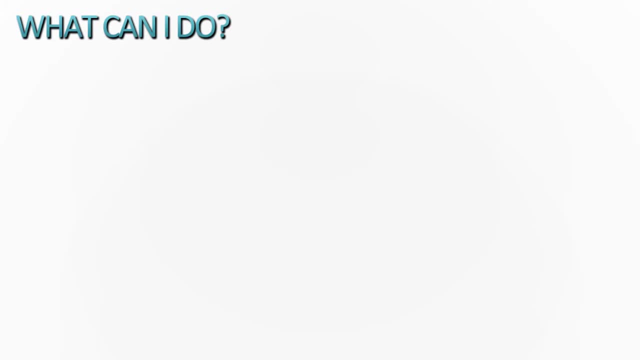 As mentioned before, it is only with detailed information that you can achieve a proper and accurate analysis to help you find the problems or the area that can be improved in your business. For the purpose of this video, we will now go a step forward into a more accurate analysis. 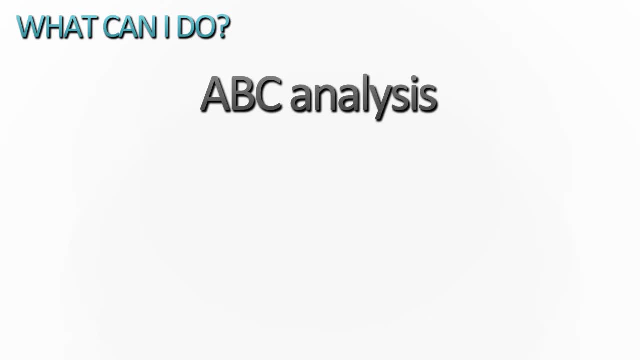 This part is commonly known as the ABC analysis or Pareto principle. So once you've discovered and examined your business trend, we now want to gather as much information as possible for each individual product or group of products, such as unit price, unit net margin, percentage, quantity sold turnover and net profit. 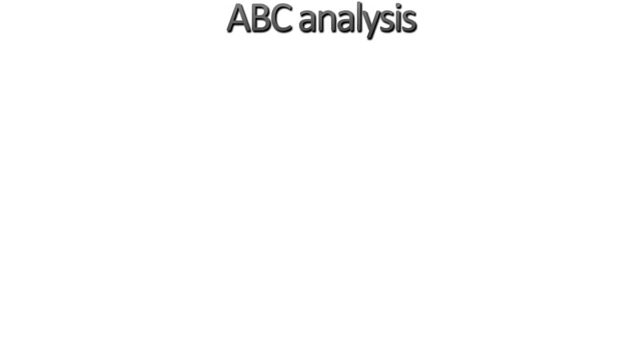 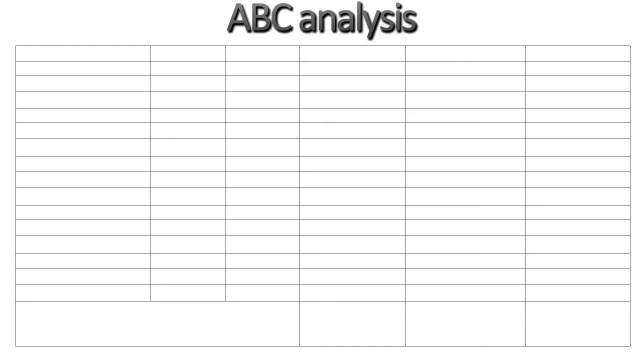 You can now place this information in a table or system as per the example on the screen. The first column will contain all your products or services. The second will have their unit prices. üç The third – their unit net margin percentage. The fourth one – their quantity sold. 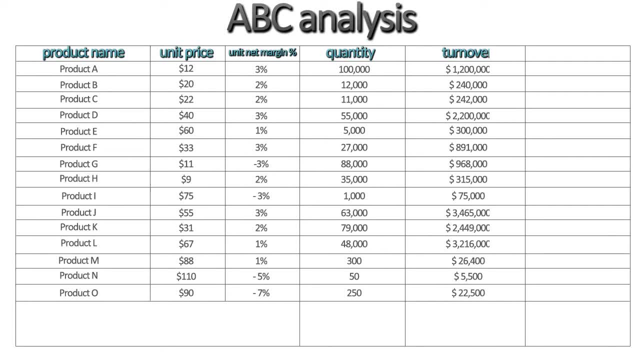 The fifth one – their yearly Total turnover. And finally, the last part: number of sold: 싶ér Wise ratio. Second – number of sold increase percentage for each unit before shopping. First – number of sold. wohl Correct of forceadtp nd percenthe krijgtki ugub 100% negative. And finally the 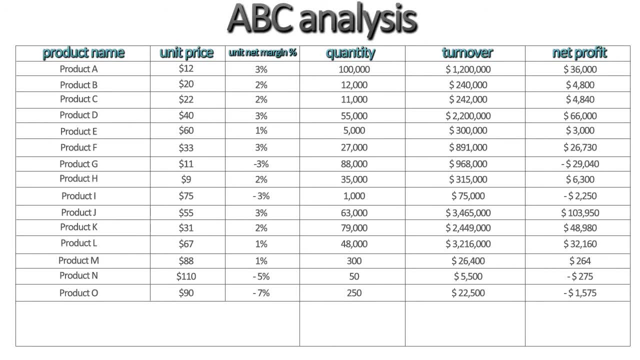 Finally, the last column will have the yearly total net profit. Next, let's calculate the total of the quantity column, the turnover and the net profit. These totals represent 100% of your business Underneath. go ahead and write 80% of that total per each column as shown on the screen. 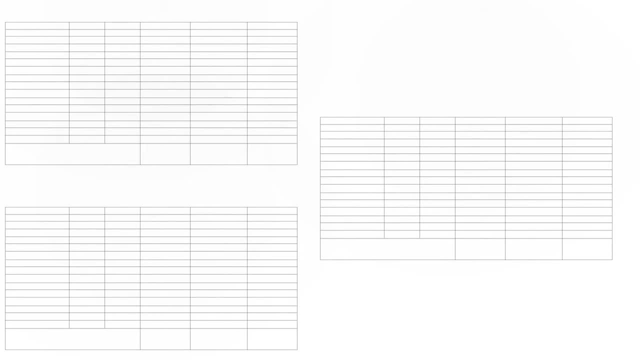 Now let's duplicate the table two more times and rename the first table A, the second one B and the third one C. Next we can sort table A by quantity, from largest to smallest, Starting from the top. let's add the figures until we reach the 80% number and draw a line. 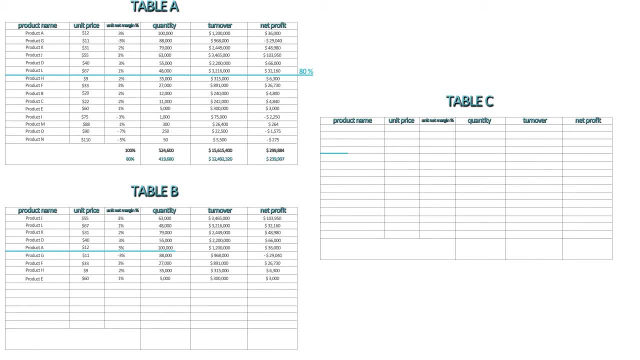 Let's repeat the same process for table B by turnover and table C by net profit. profit- okay, we now have all our products reordered by quantity, turnover and net profit and we can see that some products are above the blue line while others are below it in each table. before we begin the ABC analysis, we also need to 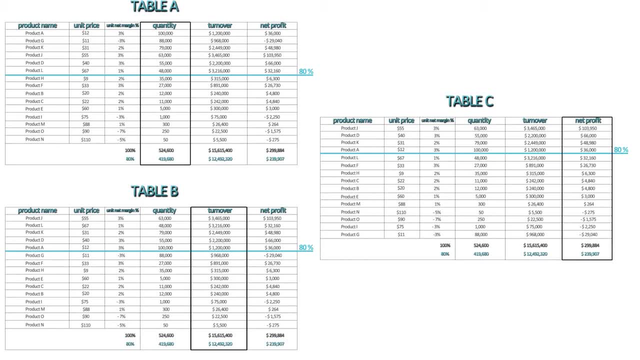 establish the priority in which we're going to analyze our products. to do so, we're going to use the color green, red and red highlighted green, which represent healthy products with low priority. red, weak ones with medium priority. and the products are highlighted in red will be the sick. 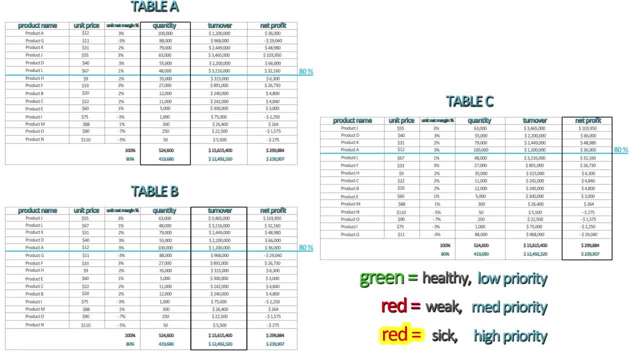 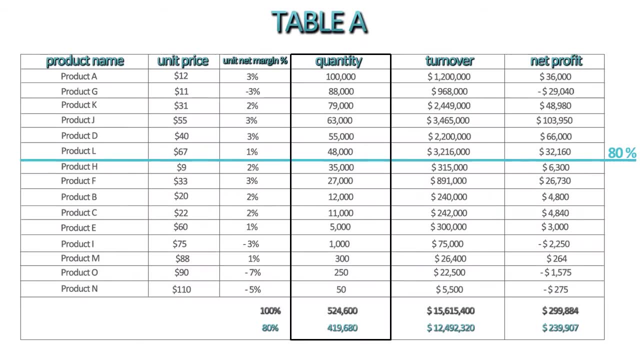 ones with high priority. we are now ready to begin the analysis, so let's examine our three tables. we can notice that in each table the product, hogy rhino here the retention rate of the production and then the maximum seedsalia in each side of the product and the stock cut into certain 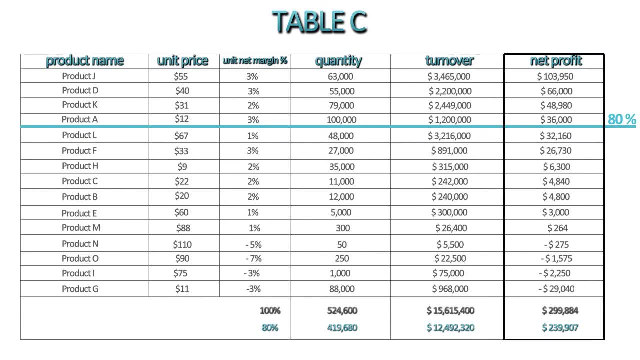 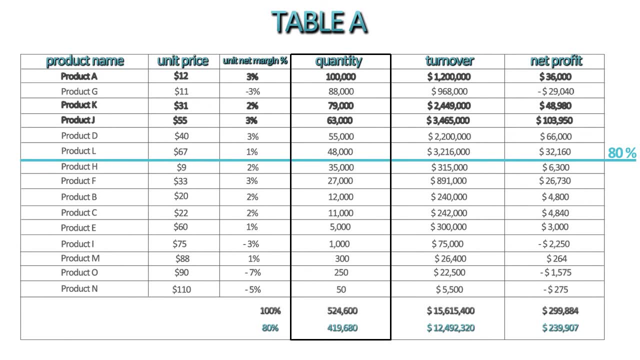 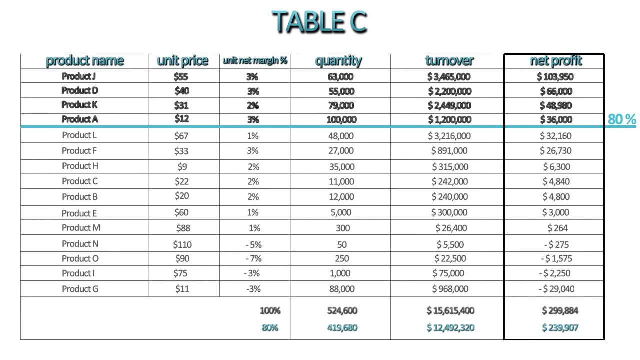 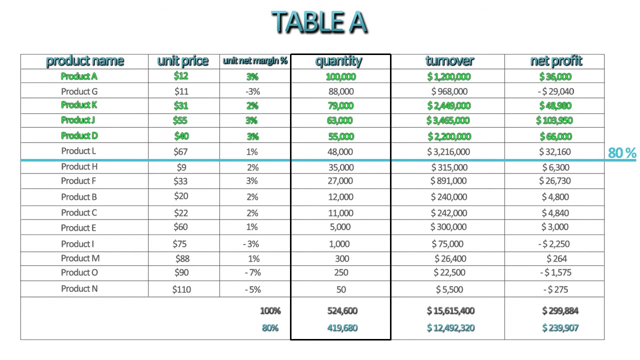 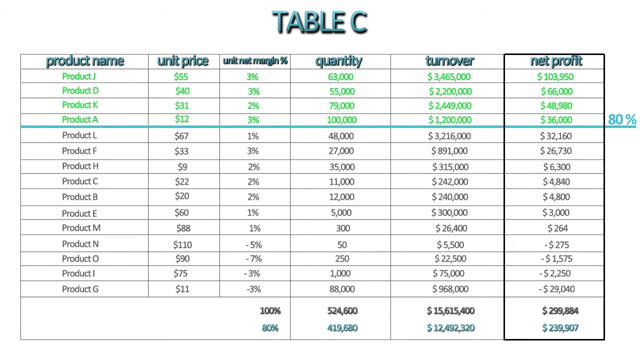 order is different, but there are similarities between some products in table A, B and C. For example, product A, K, J and D are above the line in terms of quantity, turnover and net profit, while the rest of the products are below the line. So let's go ahead and change the color to green in each table. Next we can: 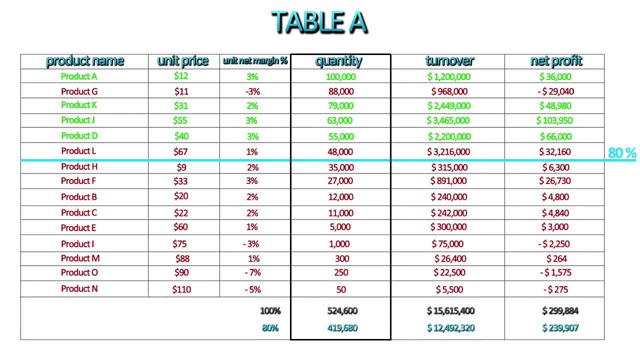 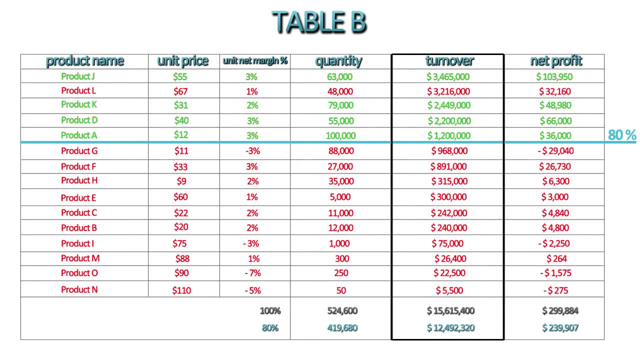 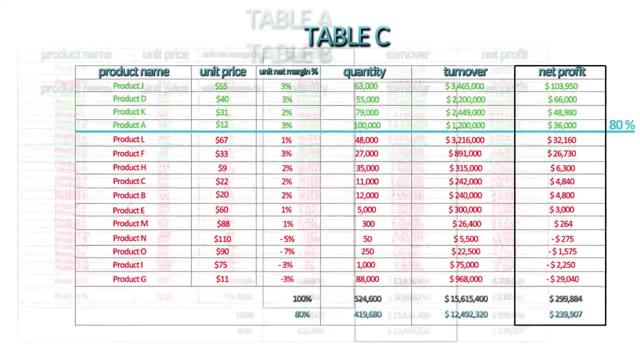 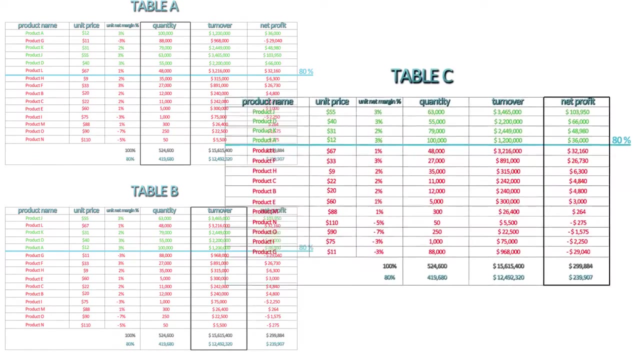 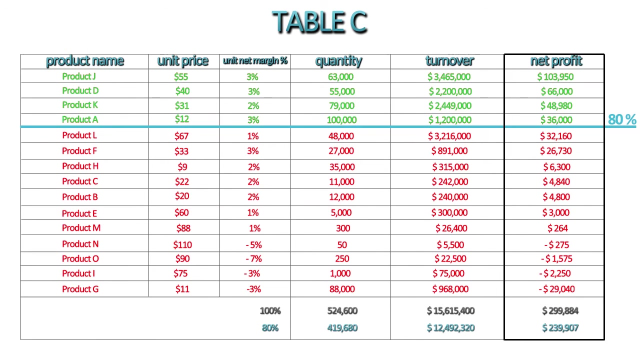 change the color of the remaining products to red, The end result should look similar to the example on the screen. Now let's examine table C. Amongst the products in red at the bottom, we can notice the product N. O, I and G are actually causing a loss to the business, So let's highlight. 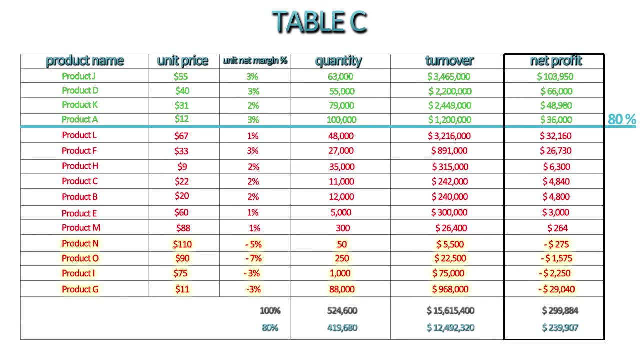 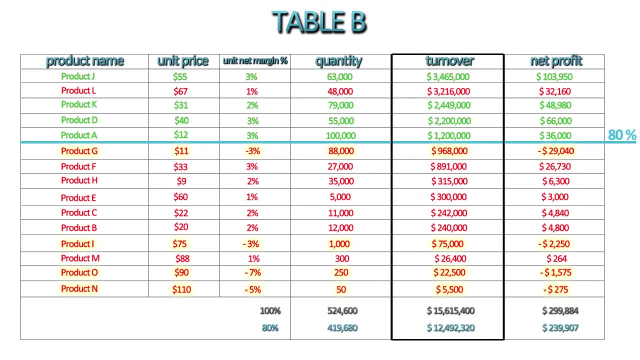 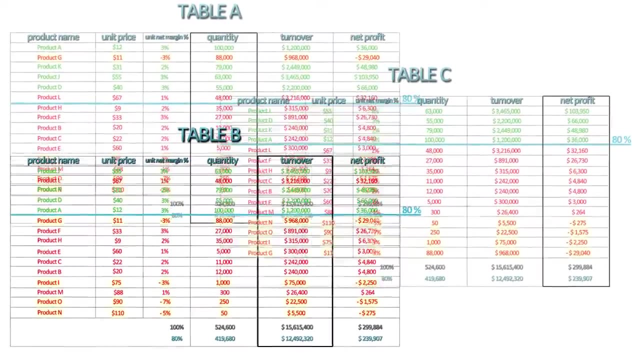 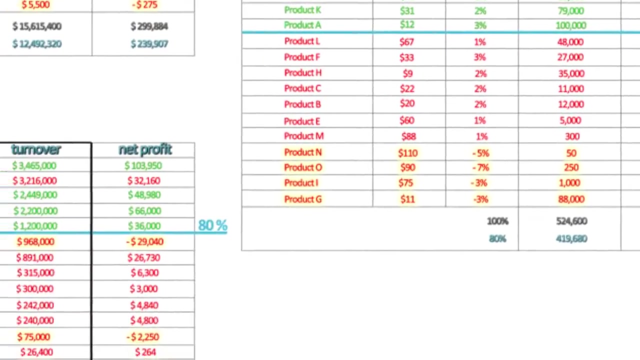 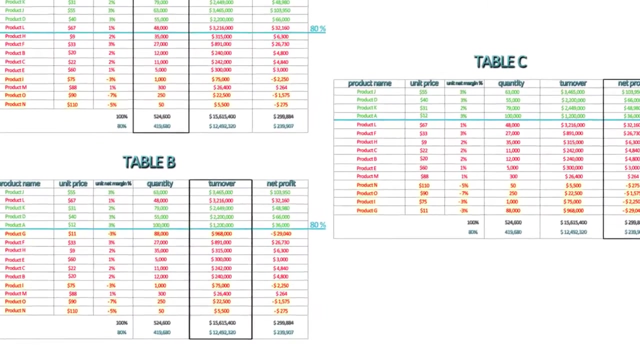 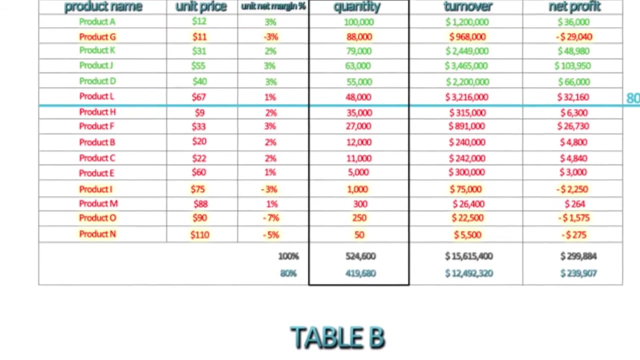 them and do the same in table A and B. Next, looking at our three tables, we can notice the product N, O and I are pretty much at the bottom of all three tables. However, product G is below the line and in table B and, as a matter of fact, it's in second place in table A. Keep in mind. 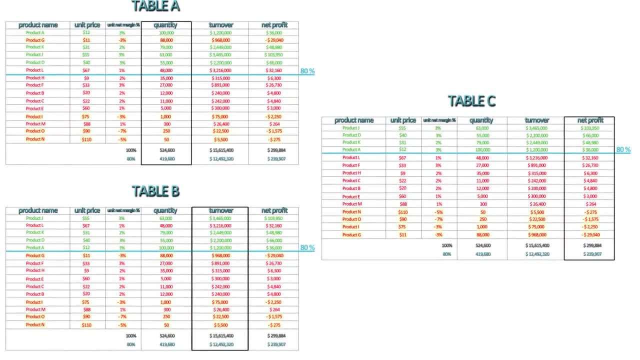 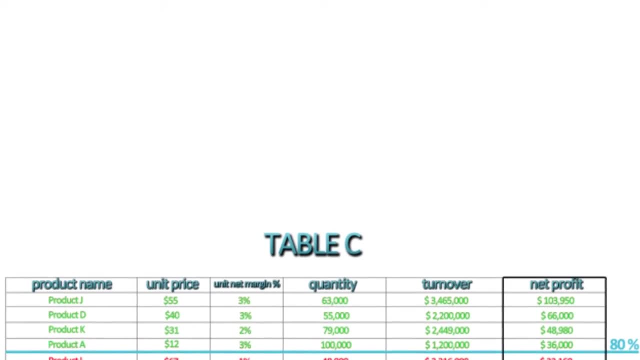 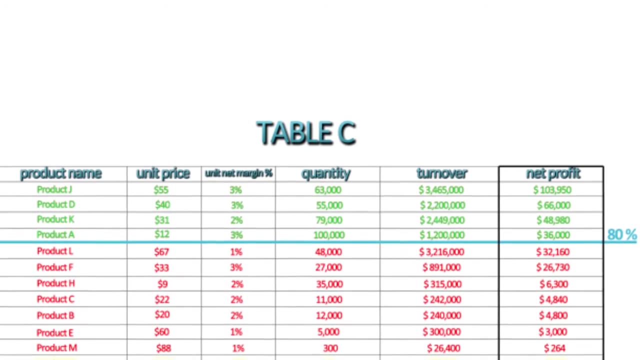 product G, as we will go back to it in a minute. As a general rule, whether your list has 10 or 100 products, you should have some in green at the top, which that consists of 80% of your sales, some in red and others highlighted at the bottom of the three tables. When a 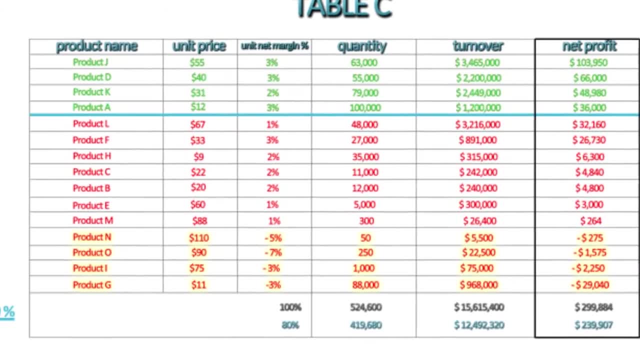 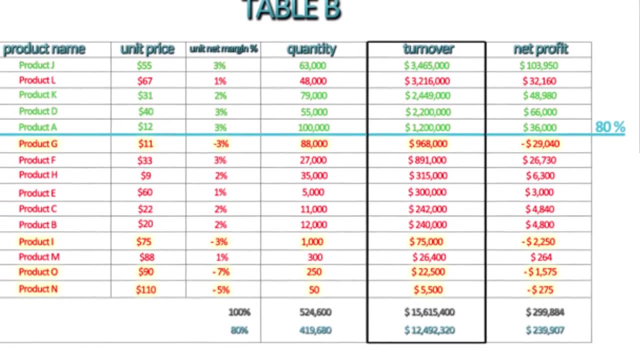 business is losing money. the products that are the top top of the table. are the products that are the top top of the table- egy Products commonly highlighted at the bottom of each table with high priority, need to be analysed first, and usually they can be eliminated or changed without affecting the business. 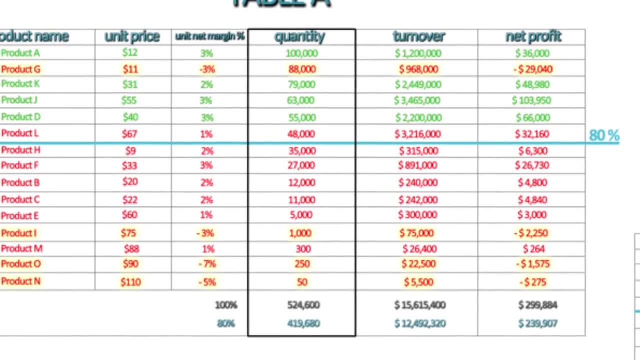 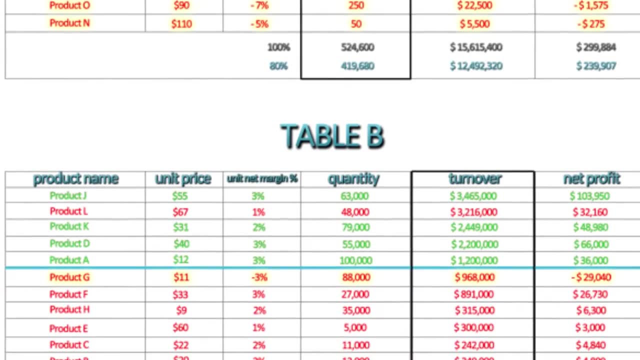 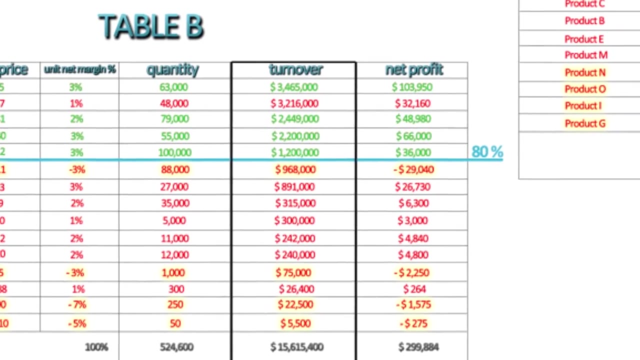 For example product N, O and I. After those, all the products in red with medium priority below the 80% margin should be analysed carefully and in detail individually. The products in green commonly at the top of each table, above the 80% margin usually. 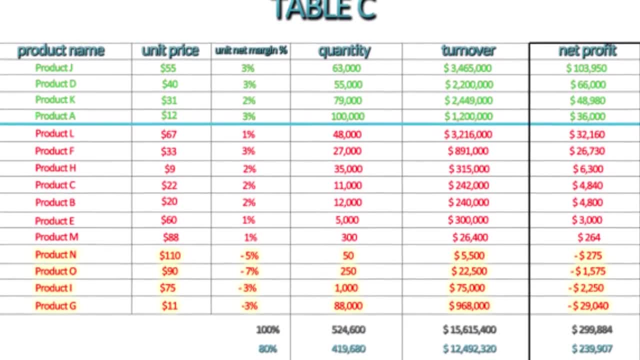 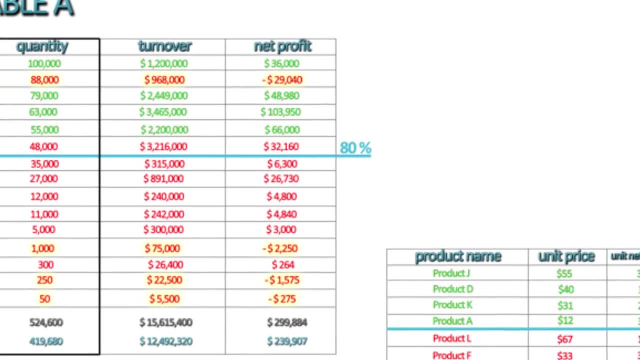 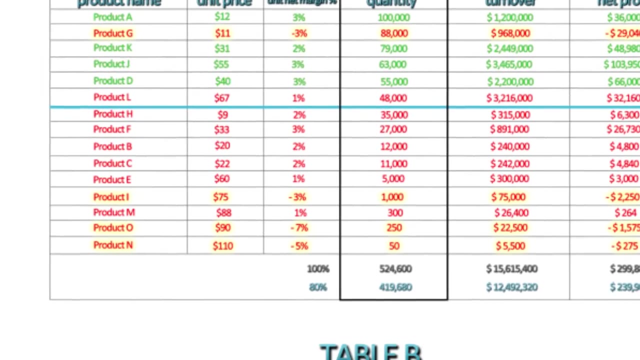 don't have any problems or don't need intervention. However, the products at the bottom, but not in all three tables, similar to product G must be analysed even more carefully. Even if G is costing the business money, its quantity and turnover are high, representing: